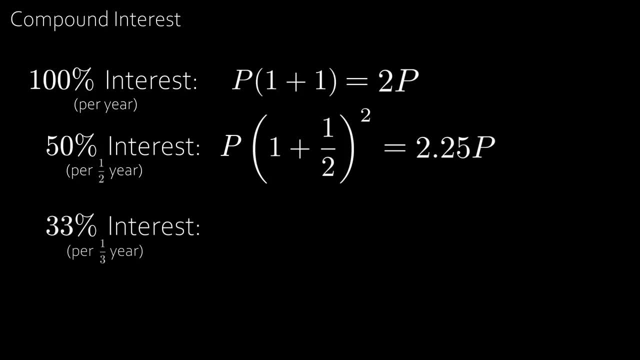 year. Now, what about 33% interest every one third of the year, or every four months? Well, we can do the same thing, but at the end of the year we end up with P times 1 plus a third. all cubed, which is equal to 2.37 times P. Now we see that this value is getting larger and larger the more times we 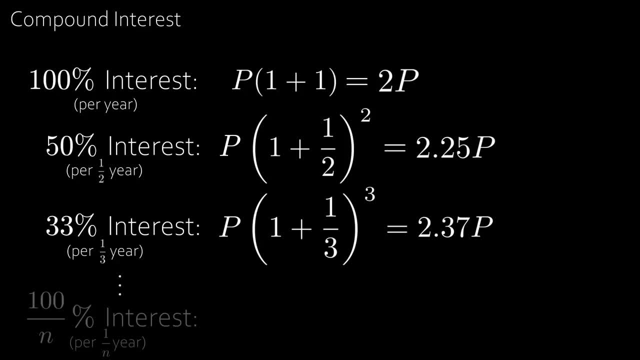 have interest imposed. Now if we kept going then we see that 100 over N percent interest every one nth of the year gives us a final value of P times 1 plus 1 over N to the power of N. And because it's getting larger and larger, we want to find the maximum value that it can be to get the most. 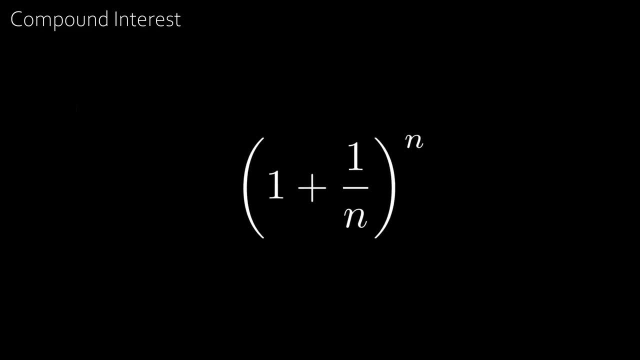 we could get. So, essentially, we want to know the limit, as N approaches infinity, of 1 plus 1 over N, all to the power of N. And actually we can calculate this number and it ends up being this irrational number: 2.71828 dot, dot, dot. and this number is famously written as the letter E, similar. 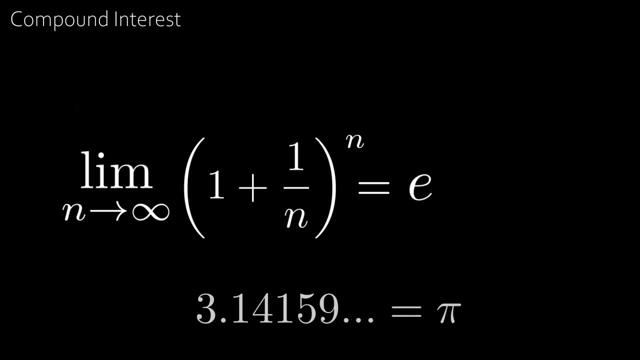 to the way that we write 3.141 dot, dot, dot as being the number pi, And E is known as Euler's constant, And what this means is that the maximum amount of interest that we have added to the amount that we could end up with is E times P, or 2.7 ish times P. Now we see that as N approaches, 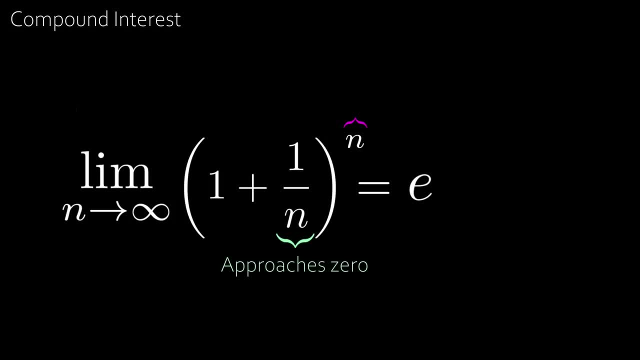 infinity. 1 over N approaches 0 and N in the exponent approaches infinity, of course. But if we make the substitution K equal to 1 over N, then K approaches 0 can replace N approaching infinity and we get the limit, as K approaches 0, of 1 plus K, all to the power of 1 over K. And this is another. 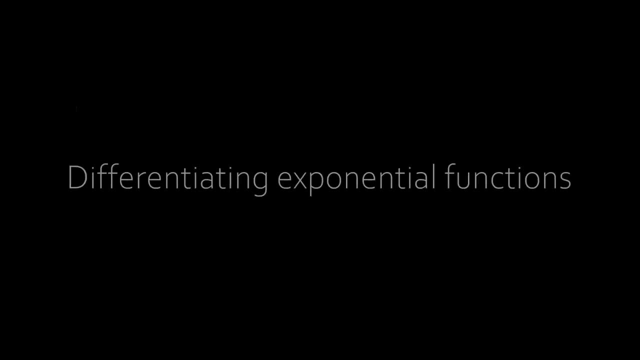 way of writing the number E. Let's now try to differentiate exponential functions. Say we had Y equal to 2 to the X. Then what is dy dx? Well, we remember that dy dx is equal to the limit as H approaches: 0 of F of X plus H minus F of X, all divided by H. Now, if we take F of X equal to 2 to 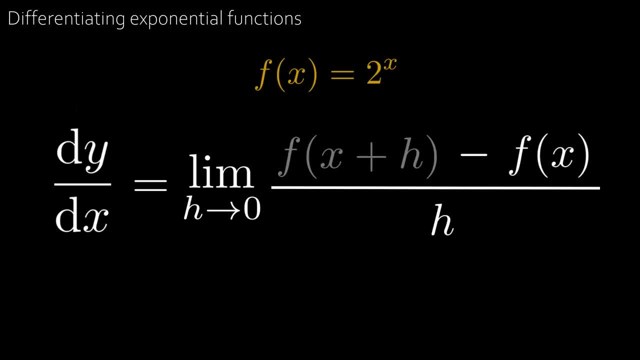 the power of X. then we have the limit, as H approaches 0, of 2 to the X plus H minus 2 to the X, all divided by H. Now, by an important rule of exponents, we can write 2 to the X plus H as 2 to the X times 2 to the H, Then factorising: 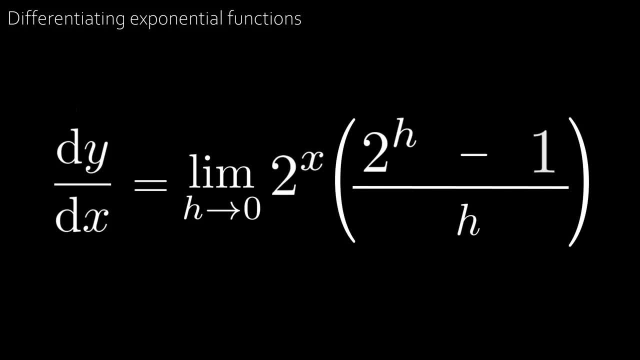 in the numerator we get 2 to the X times 2 to the H, minus 1 all divided by H. Now we can interchange 2 to the X and the limit as 2 to the X has no dependence on H. Now this limit we can. 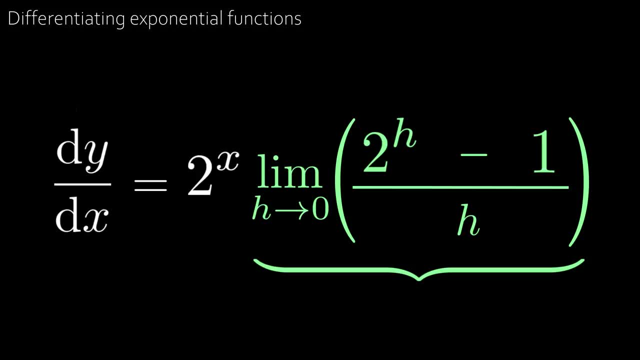 actually calculate and we get some irrational number: 0.6931, dot, dot, dot. Now this value also has a symbol, So we can write 2 to the X plus H as 2 to the X plus H as 2 to the X times 2 to the. 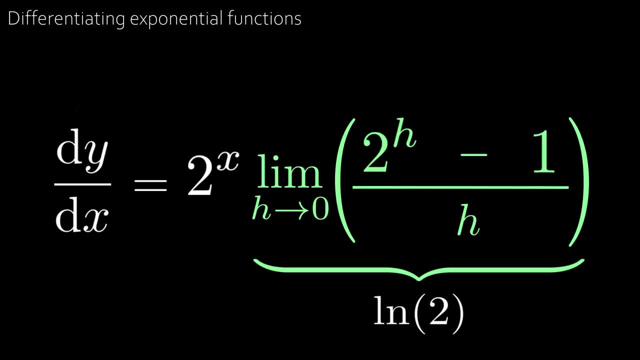 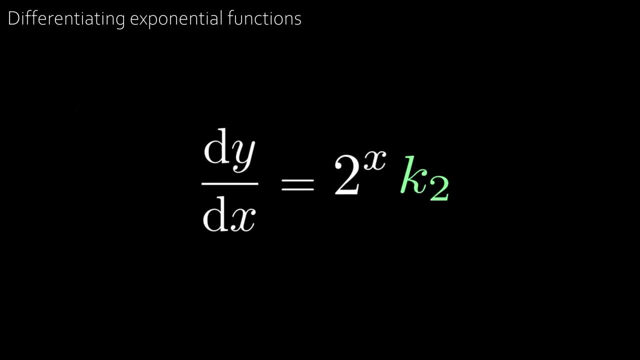 X. We took this降, see g 2, for example, which we will see later. But for now let's call this constant k2.. So dy dx is equal to 2 to the power of x times some constant k2.. Now we can do the. 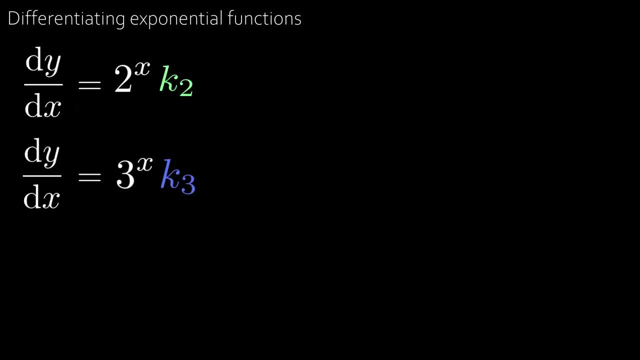 same for y equals 3 to the x, And we get dy dx is equal to 3 to the x times some other constant k3.. And for 4 to the x, we do the same thing and we get dy dx is equal to 4 to the x times some. 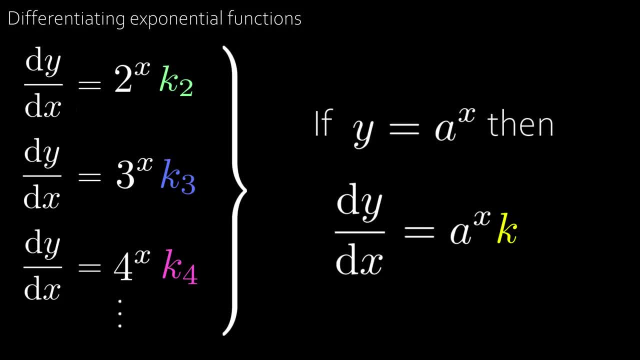 constant k4. concept k4. And we can to the x, then dy dx is equal to a to the x times some constant k. Now this is great. We found what dy dx is for exponential functions. But each time we have to calculate this constant k from scratch. 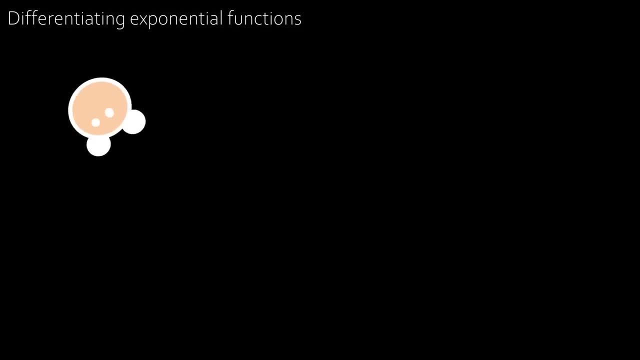 So can we make k equal to one, That is, can we find a value, a, such that if y is equal to a to the x, then dy dx is also equal to a to the x. Well, we know that we can write dy dx as a limit, and we: 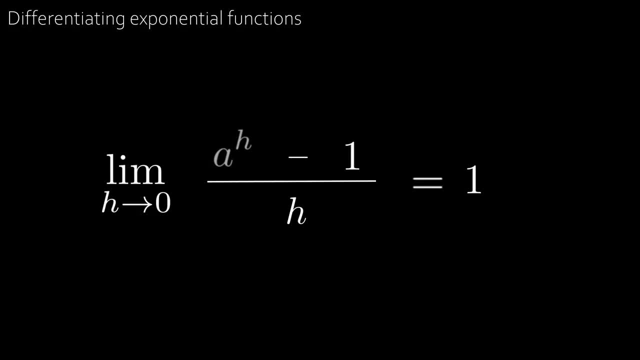 can then divide both sides by a to the x, And we see that this left side is actually our constant k from before. So we want our value k to be equal to one. So now, what value of a should we choose? Well, let's try a equal to e, Euler's constant, And we remember that e is equal to the limit. 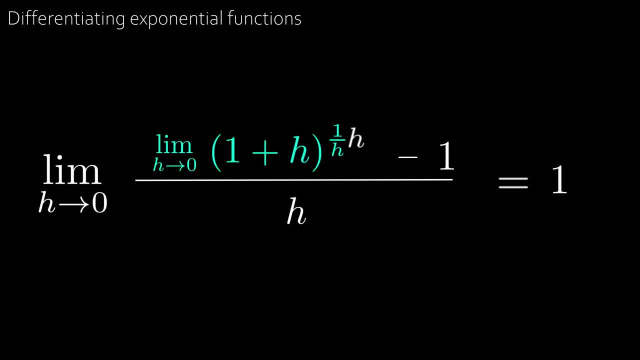 as h. So we can then write dy dx as a limit as h approaches zero of one plus h, all to the power of one over h. Now we don't need to write the same limit twice And we see that h cancels in the exponent. Then 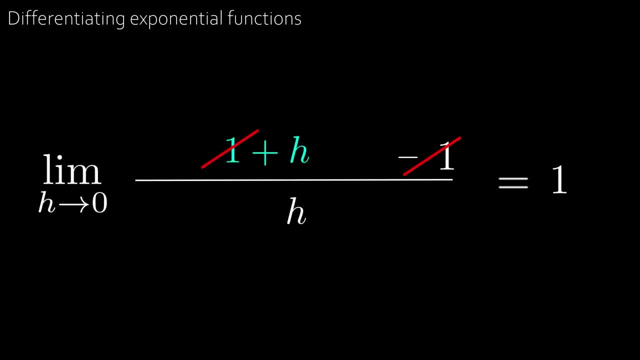 the ones, cancel in the numerator, leaving the limit, as h approaches zero, of h over h. And we know that h over h is just one, And since there are no h's left, we can remove the limit and we get one. This means that if y is equal to e to the x, then dy, dx, is also equal to e to the x. 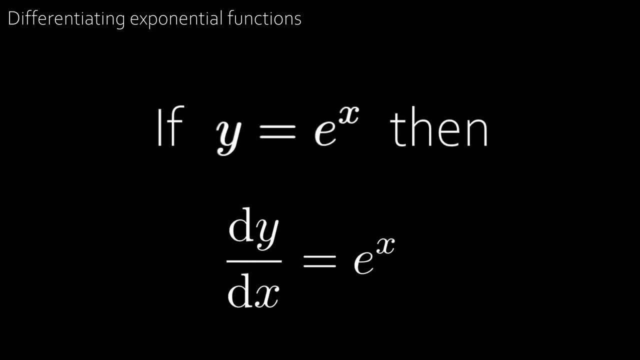 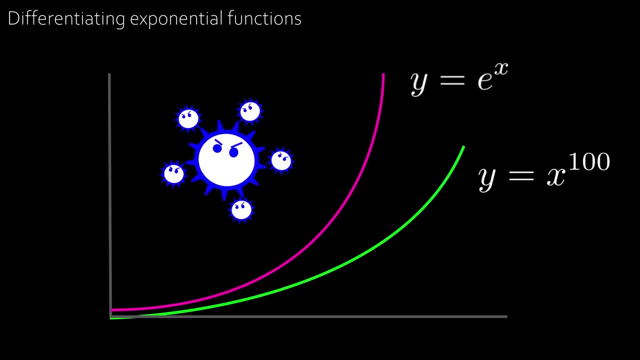 And because the derivative is itself. this makes y equal e to the x, one of the fastest growing functions in mathematics, And in fact it's scarily quick, because this means the spread of infectious diseases is extremely fast and only gets faster. Now let's take a look at one of the slowest functions in mathematics, And it's very related. 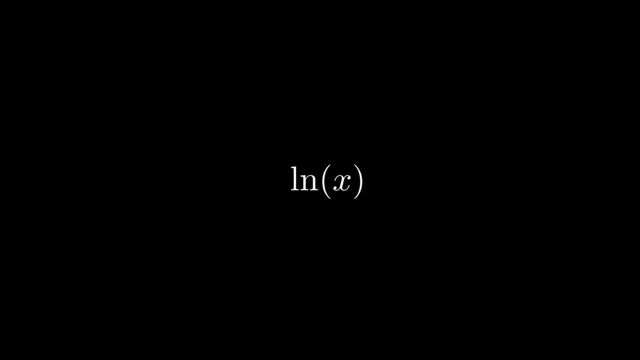 to one of the fastest functions in mathematics, And that function is known as the natural function, Logarithm. Now we know that two squared is equal to four and two cubed is equal to eight, But two to the power of what is equal to six. Now we can write this number as log base: two of six. 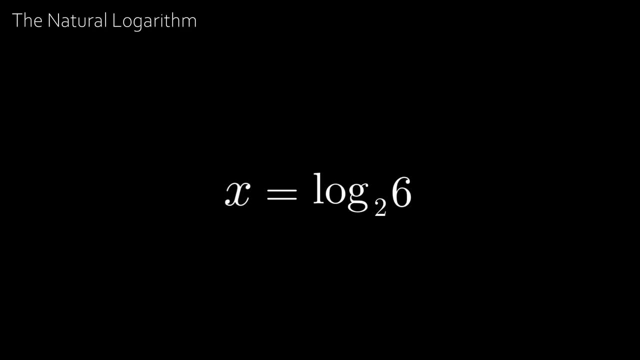 where log base two is a function. And to see how we get this function, let's consider y equal to log base two of x. Now we have a graph of y is equal to two to the x And if we reflect this graph in the line y equals x, then we get the inverse function: y equals two. 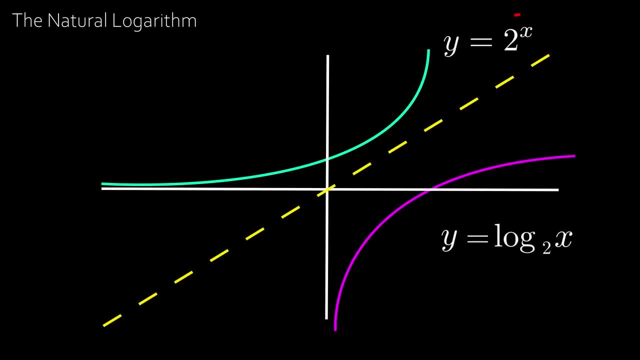 Y equals log base two of x. Now let's replace two to the x with e to the x, And remember, e is a number. two point seven, one, eight, two, eight, dot, dot, dot. Then it's reflection in y equals x becomes y equal to log base e of x. Now, log base e of x is famously written as ln x, which stands: 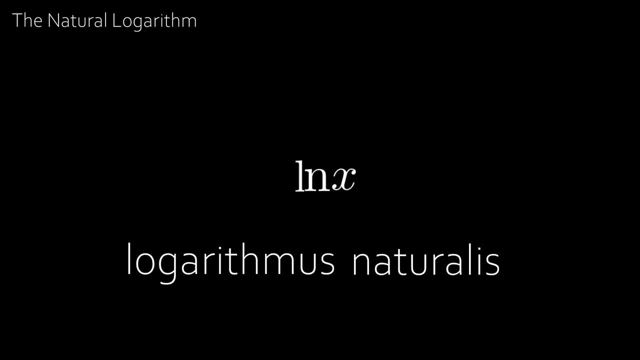 for logarithmus naturalis, which is Latin for natural logarithm. Now logarithms have some very important functions. They're called logarithms of natural logarithm. Now logarithms have some very important functions. They're called logarithms of natural logarithm. Now logarithms have some. 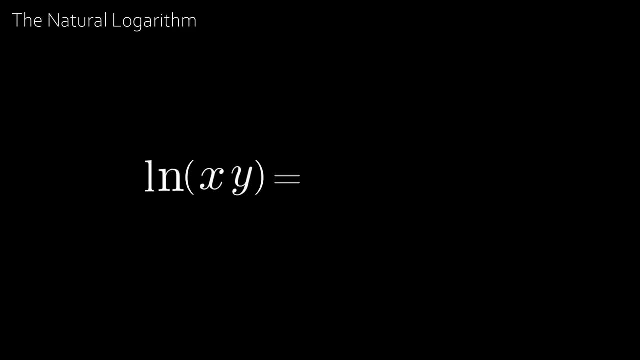 very important properties, Namely: the logarithm of a product is the sum of logarithms, which also implies that ln of x to the k is equal to k, ln x. And since exponentials and logarithms are inverse functions, then e to the ln x is equal to x. Now, with this, we can also see that ln of x divided by 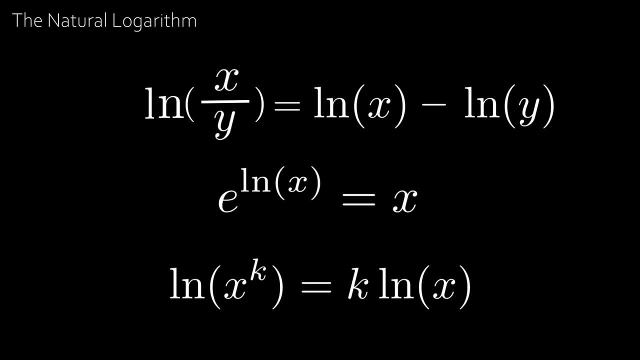 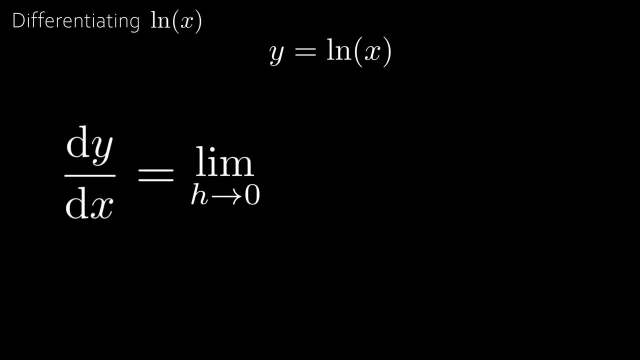 y is equal to ln x minus ln y. Now the natural logarithm is one of the most important functions in mathematics and we can start to see its usefulness when we differentiate it. So take y equal to ln x and we know that dy dx is equal to the limit as h approaches zero of f, of x plus h. 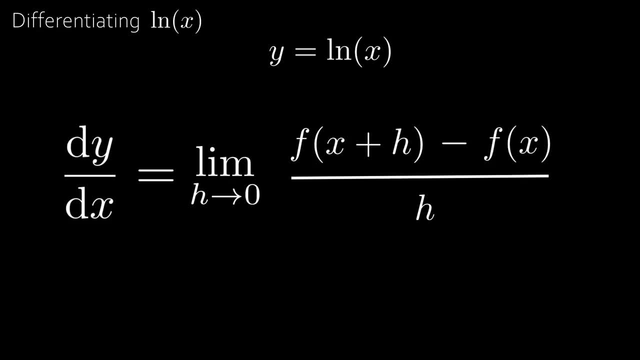 minus f of x, all divided by h, And substituting in, we get ln of x plus h minus ln x in the numerator. And now from one of the properties we can rewrite the numerator as ln of x plus h divided by x. And let's write this: divided by h. 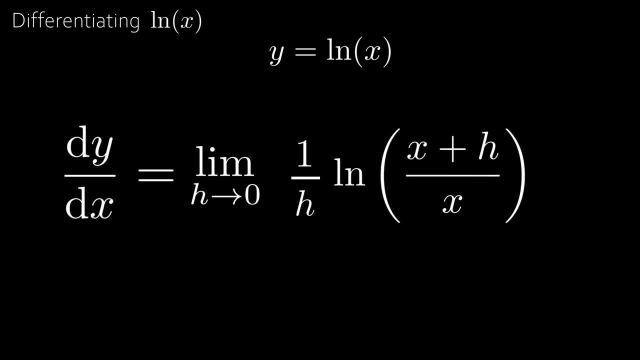 to the side as 1 over h, And we know from another property that we can bring this 1 over h to the exponent. Now we see here that x cancels, which leaves us with 1 plus h over x, And similarly to: 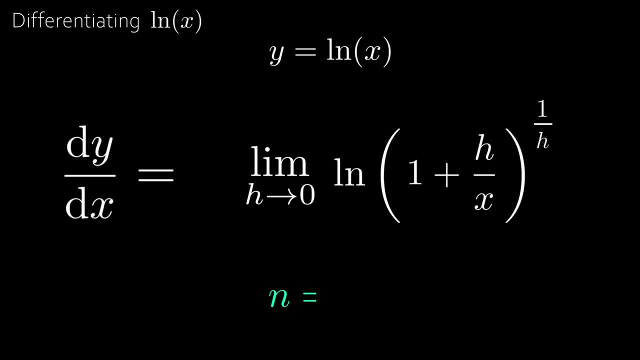 before let's make the substitution n equal to h over x. So first we change the limit as h approaches 0 to the limit as n approaches 0, because when h approaches 0, n also approaches 0. And then we have 1 plus n. 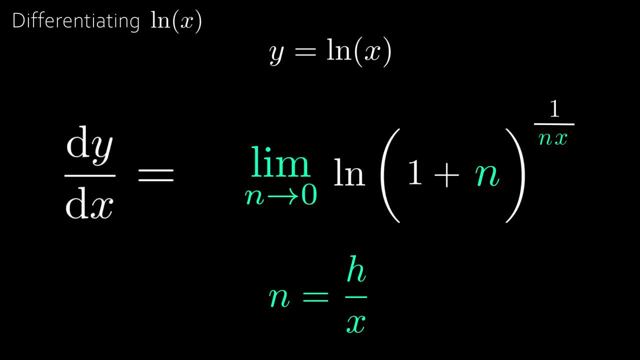 in the bracket and 1 over nx in the exponent. Now we can write 1 over nx as 1 over n times 1 over x, And by one of the logarithmic properties again we can bring 1 over x to the front. Now 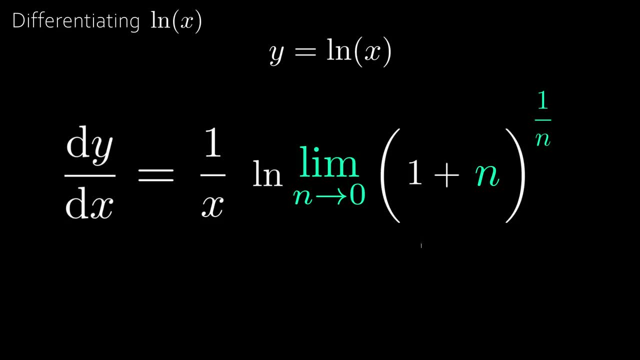 we can swap the limit and natural logarithm and we see that this part here is our number, e, And since ln of e is equal to 1, we have that when y is equal to ln of x, dy, dx is equal to 1 over. 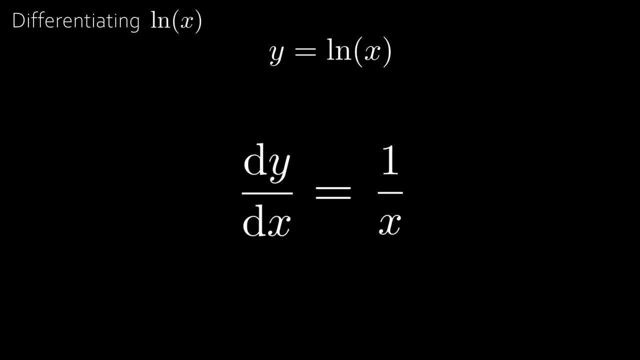 x, And this unbelievable connection has very important consequences. For example, if any of you have done integration, then you know that you cannot calculate the integral of 1 over x- dx the normal way, But here we show that this value is equal to ln of x. Now this relation also is the 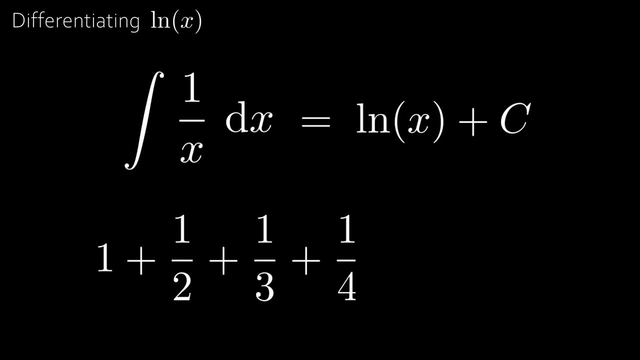 reason why the harmonic series, which is the sum of all 1 over n, diverges to infinity. And a very trick is that we can write a to the power of x as e to the ln of a to the x, which is just e to.